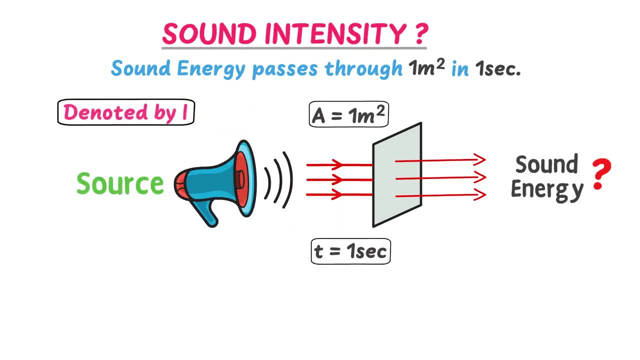 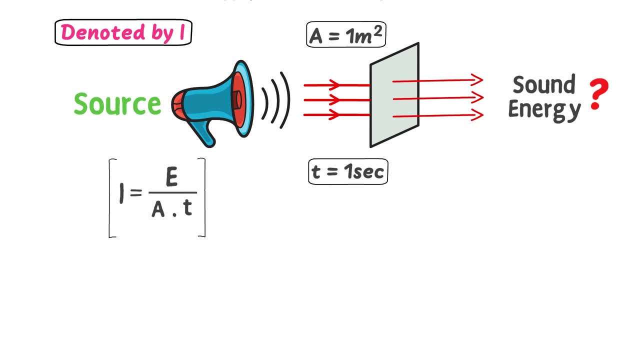 Sound intensity is denoted by I. Mathematically, we write it: I is equal to E upon A into T, where E is the sound energy that passes through unit area, or 1 meter squared area, A and time, T is equal to 1 second. 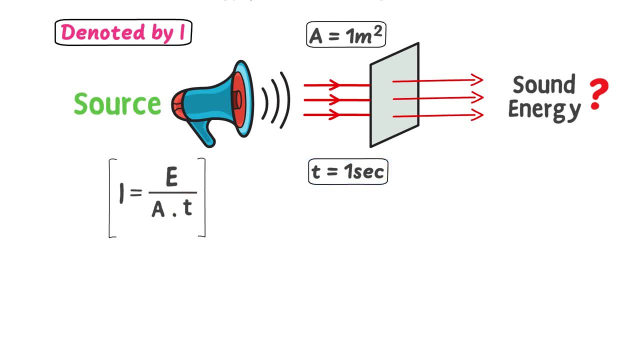 What about the SI unit of sound intensity? Well, we know that the SI unit of energy is joule, The SI unit of area is meter squared and the SI unit of time is second. So the SI unit of sound intensity is joule per square meter per second. 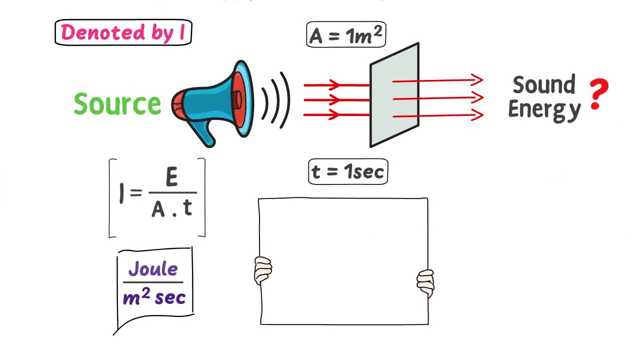 We can also write another equation of sound intensity in terms of power, For example. we know that power is energy or work done per second, or P is equal to E upon T. Now, instead of this E upon T, we will plug in this equation as simply the power. 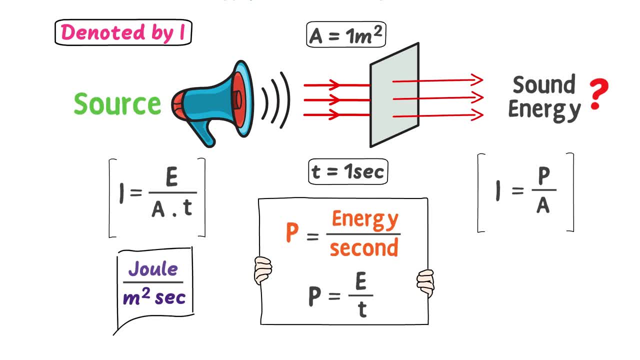 Thus we get I is equal to P upon A. We know that the SI unit of power is watt and the SI unit of area is meter squared, So we get to watt per square meter. Therefore, note it down that we have two equations for sound intensity. 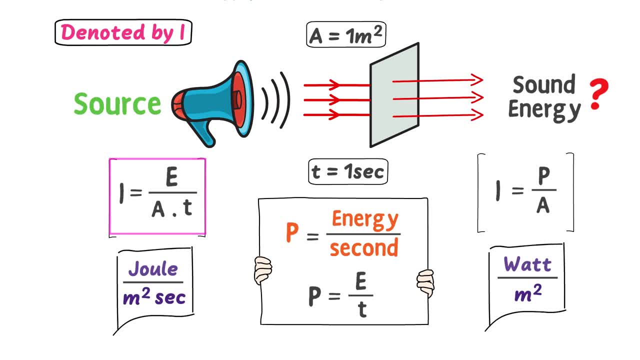 I is equal to E upon A into T, or I is equal to P upon A, And we have SI units like joule per square meter per second or watt per square meter. Mostly we use this SI unit, watt per square meter, for sound intensity. 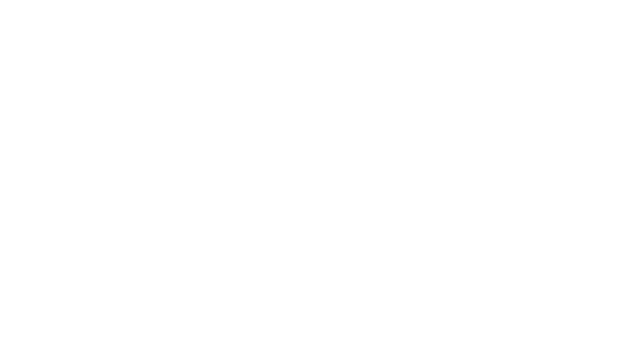 Now understanding sound intensity. we know that sound waves are different points from a source. Let's consider a point source. S produces sound. We know that sound waves are sound. energy spreads in a spherical way in all directions as they move away from the point source. 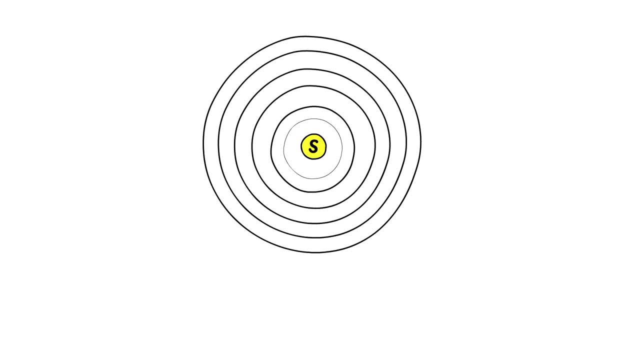 Now I am interested to find the sound intensity at point X and at point Y. Now sound intensity at point X is I is equal to P upon A, And also sound intensity at point Y is I is equal to P upon A. 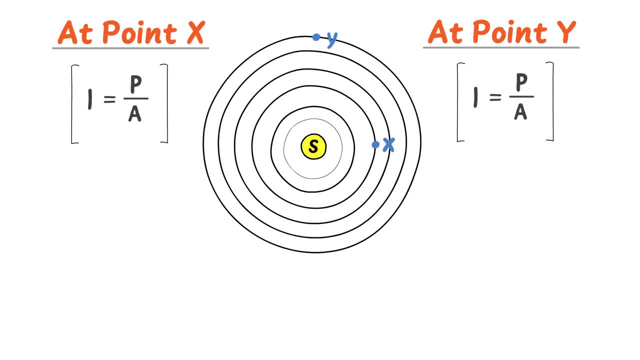 Now listen carefully. Sound energy are sound waves spread in three-dimensional ways: spherically, We know that the surface area of sphere is 4 pi R squared. So the equation of sound intensity at point X can be written as I is equal to P upon A. 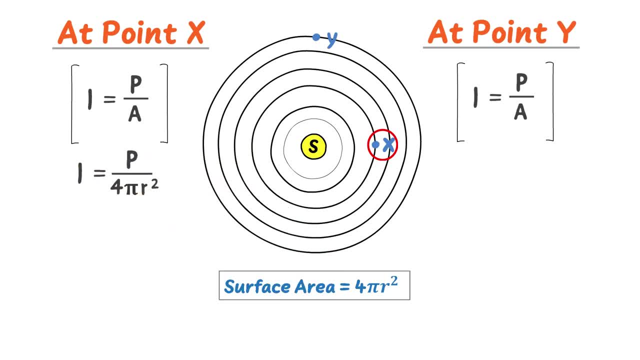 I is equal to P divided by 4 pi R squared. Also, the equation of sound intensity at point Y can be written as: I is equal to P divided by 4 pi R squared. The distance of point X from the source is R. 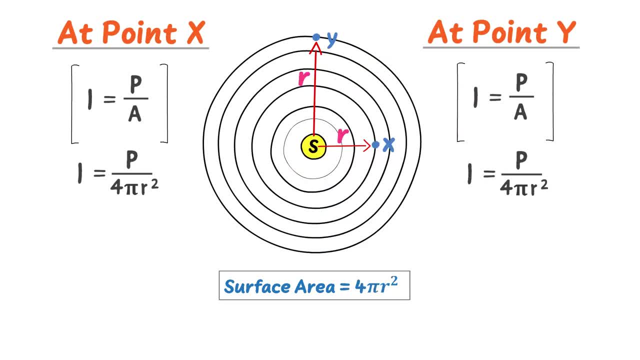 And the distance of point Y from the source is also R. Now, according to this equation, intensity is inversely proportional to the square of radius. The distance, or radius R of the point X from the source is small, So the sound intensity will be high at point X. 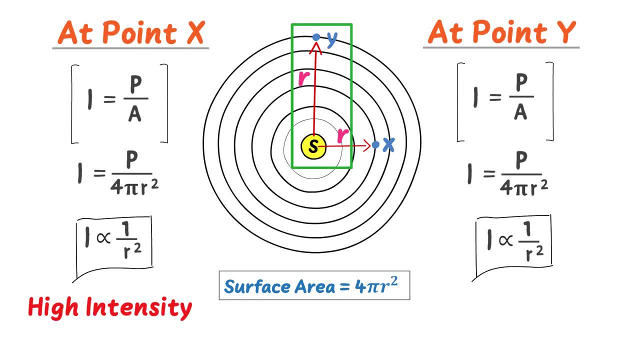 While the distance or radius of the point Y is large, So the sound intensity will be low at point Y. Thus, moving away from the source means larger radius. Larger radius means less intensity, and vice versa. Therefore, remember that sound intensity at point X is high. 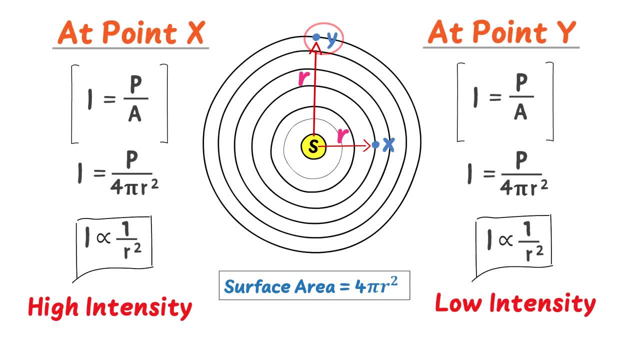 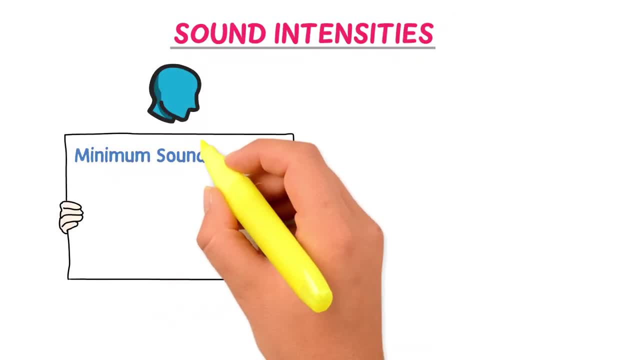 And sound intensity at point Y is low. Finally, let me teach you about different intensity levels. The minimum sound intensity or lowest sound intensity human ear can hear or detect is: I naught is equal to 10 raised to the power negative 12 watt per meter squared. 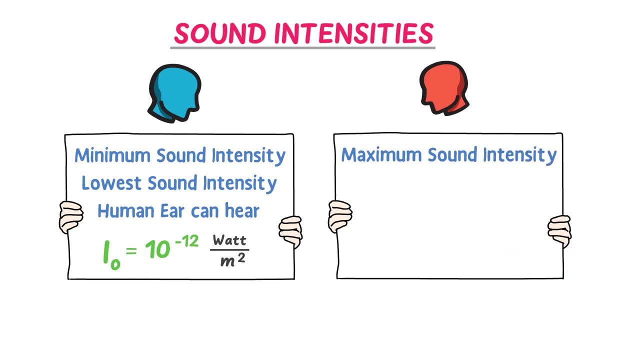 Secondly, the maximum sound intensity, or highest sound intensity human ear can hear or detect, is I is equal to 1 watt per meter squared. Thirdly, the sound intensity- 1000 watt per meter squared- can rupture or destroy your ear drums. This was all about sound intensity.